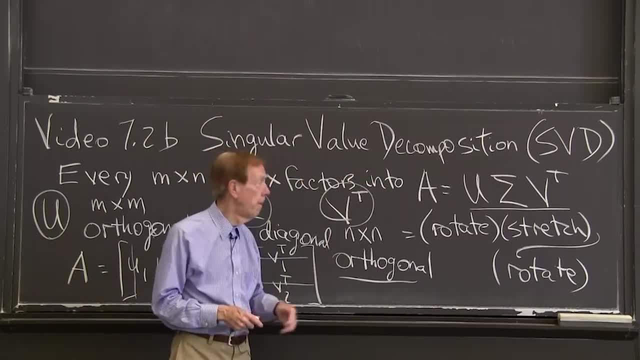 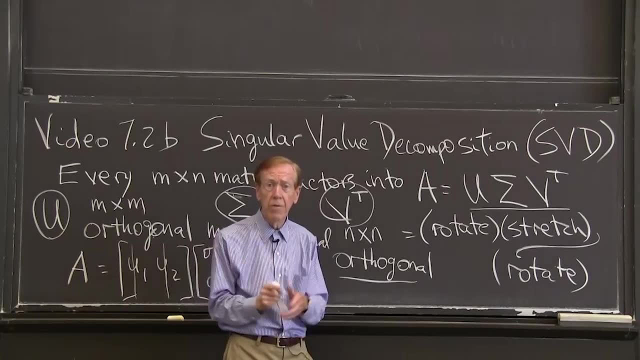 What's the difference between this SVD, this, this and the v lambda v- transpose, v inverse, v lambda v- inverse for diagonalizing other matrices. So the lambda is diagonal and the sigma is diagonal, but they're different. 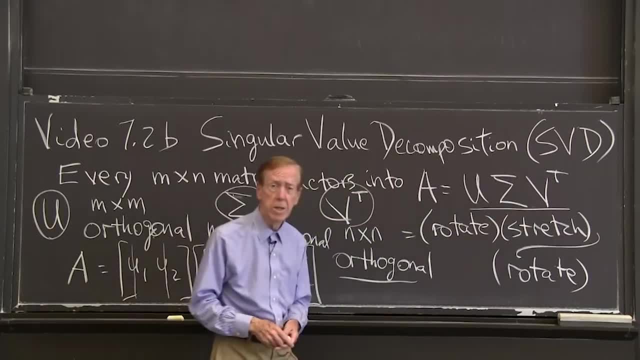 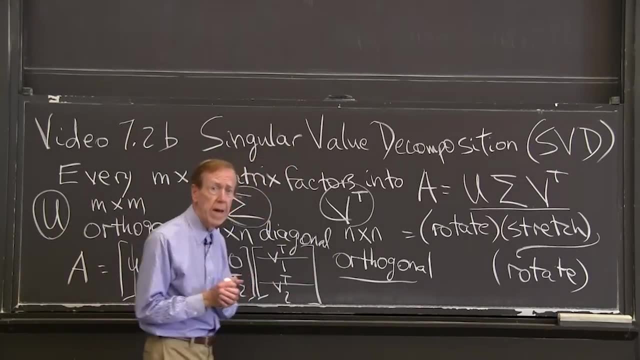 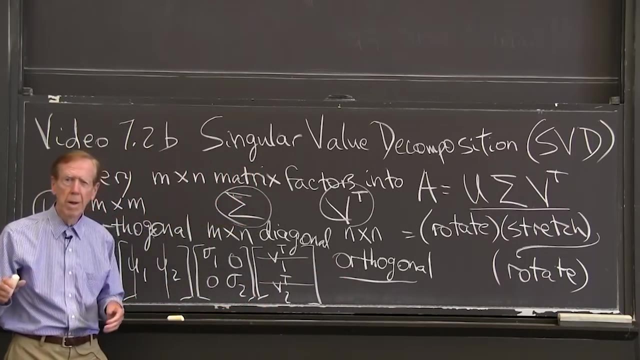 The key point is I now have two different matrices, Not just v and v inverse, but two different matrices. But the new great advantage is they are orthogonal matrices Both of them. So by going to and I can do it for rectangular matrices also. 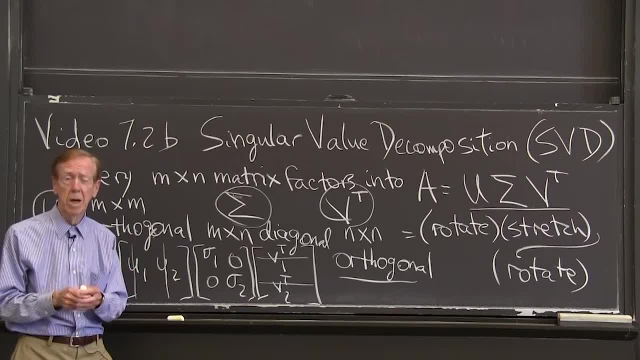 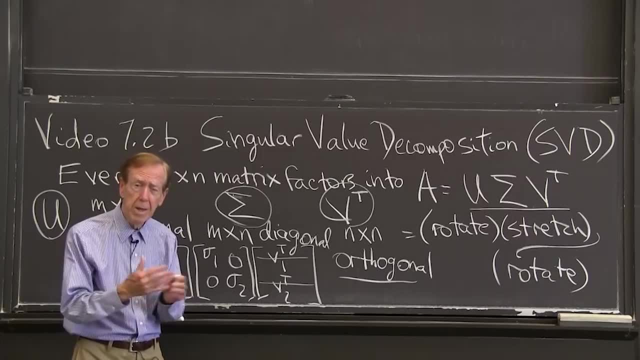 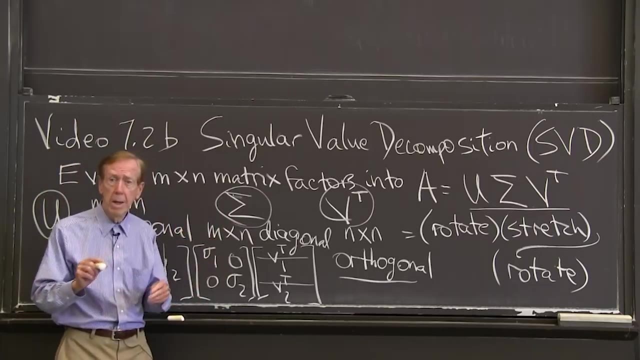 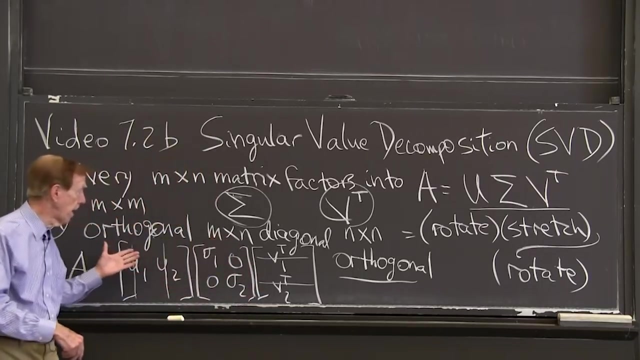 Eigenvalues really worked for square matrices. Now we really are. we have two. We have an input matrix and an output matrix, And those spaces m and n can have different dimensions. So by allowing two separate bases we get rectangular matrices and we 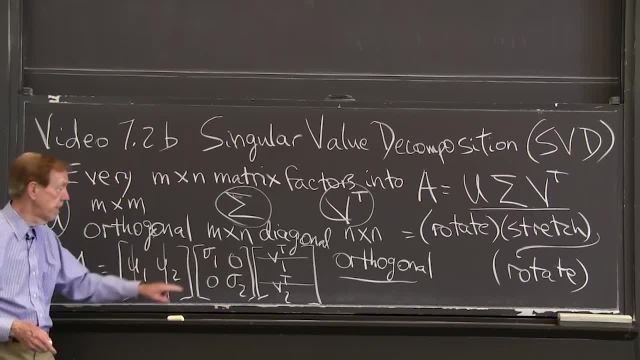 get orthogonal factors with again a diagonal, And this is called these numbers sigma. instead of eigenvalues are called singular values. So these are the singular values, These are the singular vectors, The right singular vectors and the left singular vectors. 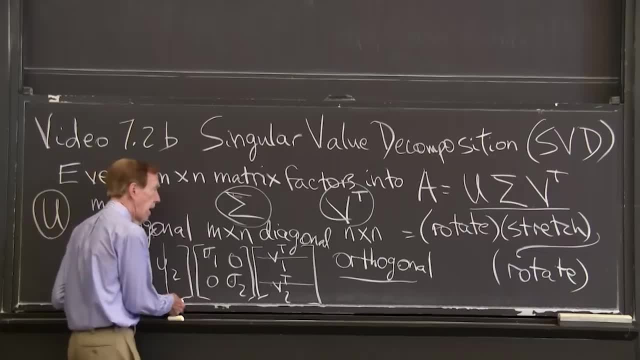 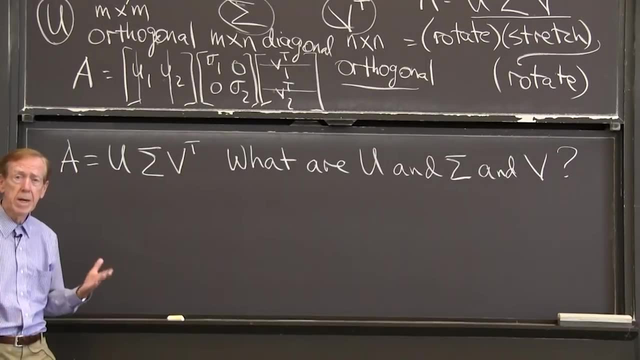 That's the statement of the factorization. But we have to think a little bit. What are those factors? What are the? can we see how, why this works? So I want that And let me do as you see this coming. 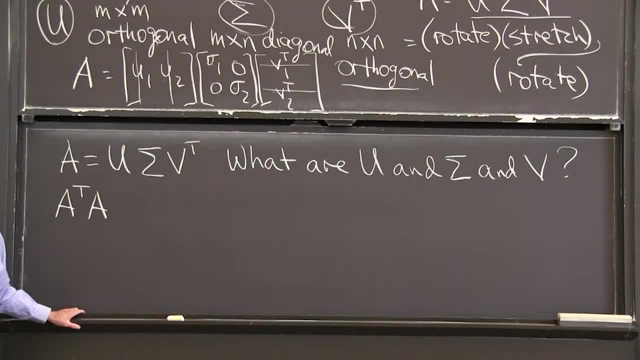 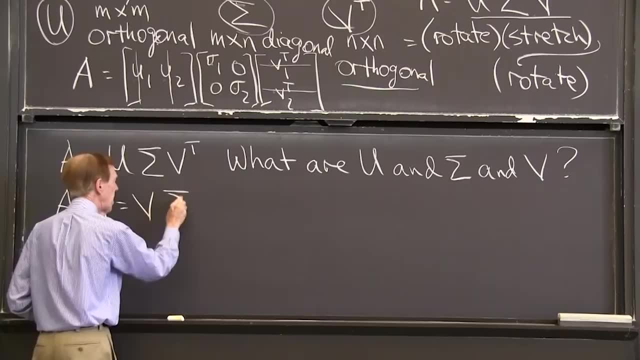 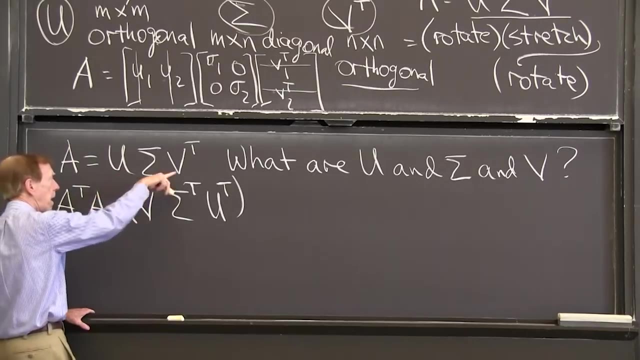 I'll look at A transpose A. I like A transpose A. OK, so A transpose will be. I transpose this: v sigma transpose, u transpose, right, That's A transpose. Then I multiply by A: u sigma v transpose. And what do I have? 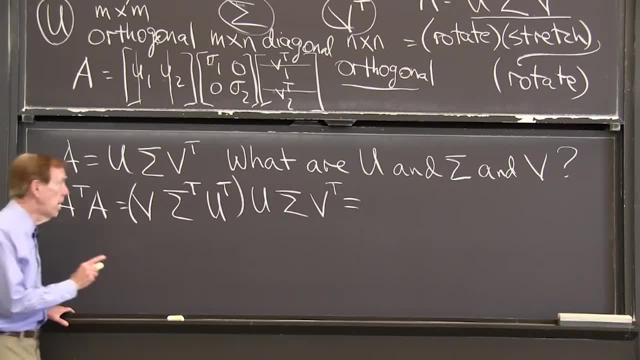 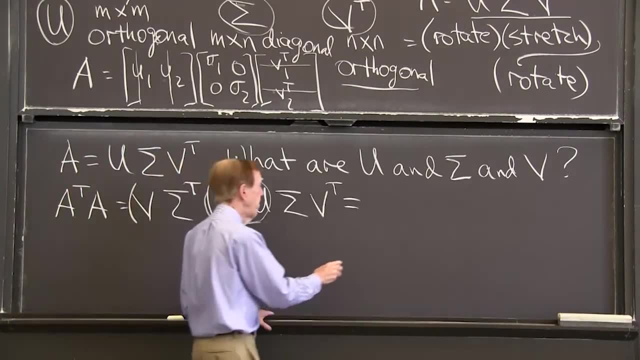 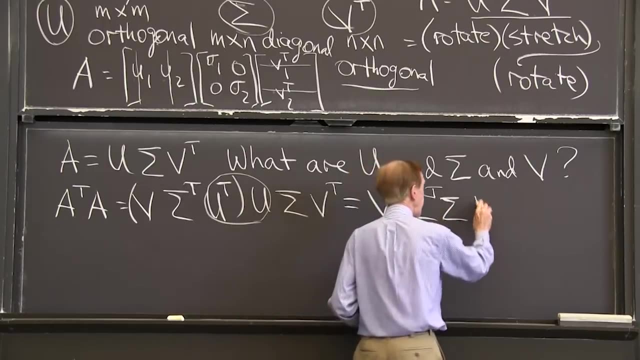 Well, I've got six matrices, But u transpose u in. here is the identity because u is an orthogonal matrix. So I really have just the v on one side, a sigma transpose- sigma that'll be diagonal and a v transpose on the right. 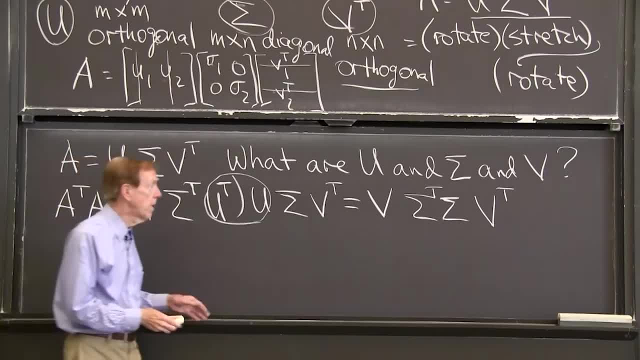 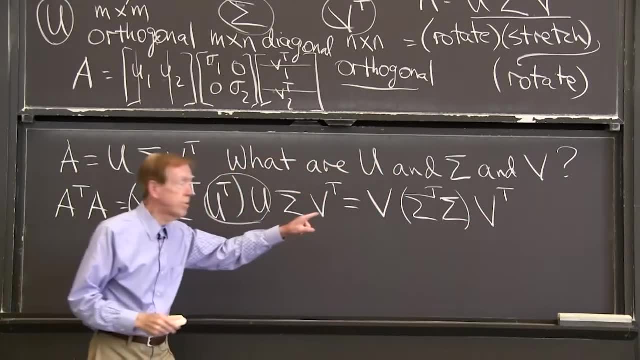 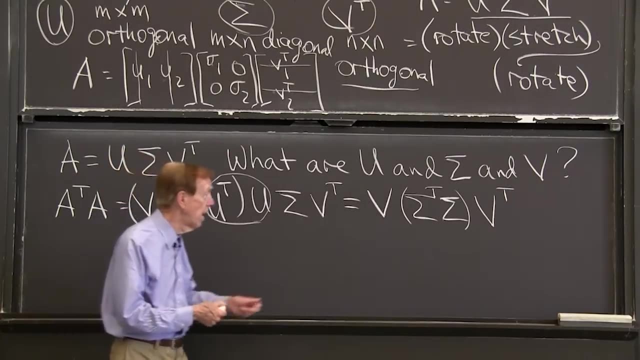 Oh, this, I recognize, This, I recognize. Here is a single v, a diagonal matrix, a v transpose What I'm showing you here. what we reached is the eigenvalue, the diagonalization. the usual eigenvalues are in here. 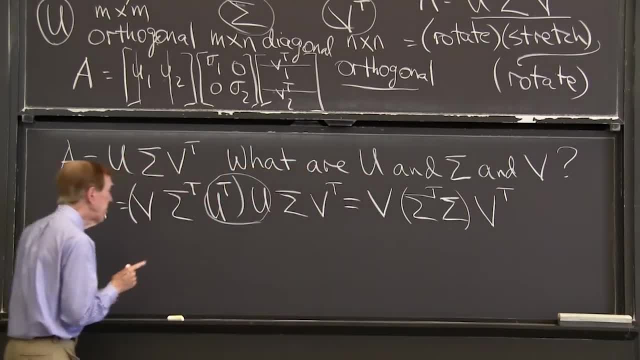 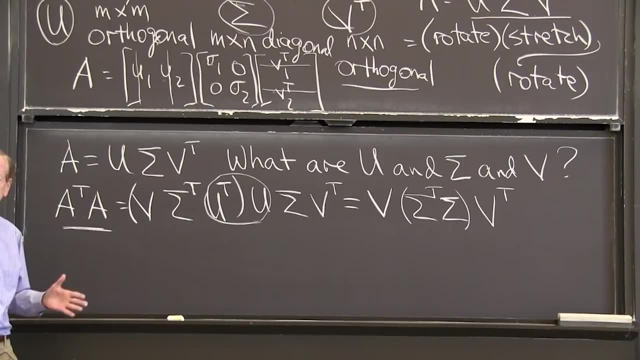 and the eigenvectors are in here, But the matrix is A transpose A. Once again, A was rectangular and completely general and we couldn't see perfect results, But when we went to A transpose A, that gave us a positive, semi-definite matrix. 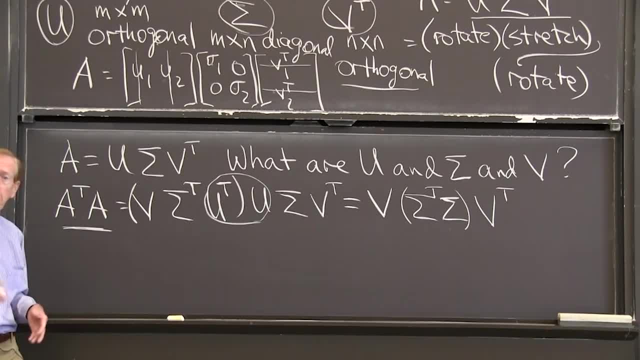 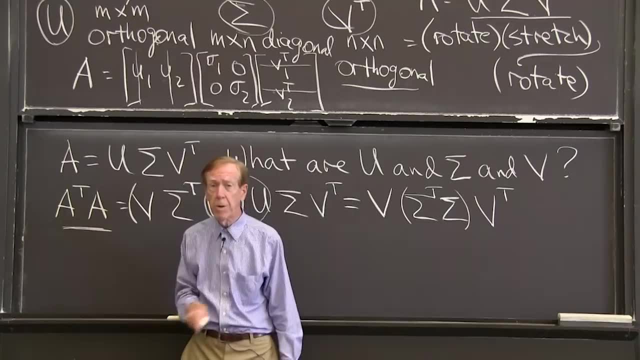 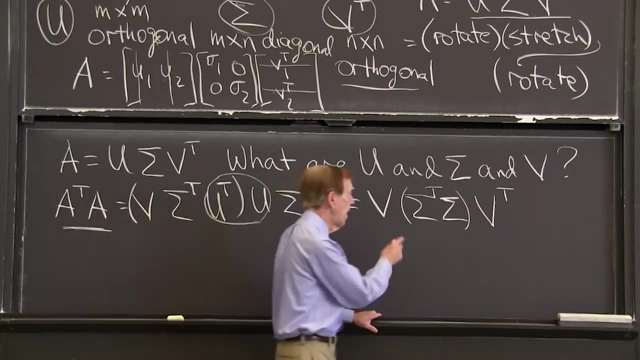 symmetric for sure, Its eigenvectors will be orthogonal. That's how I know This v matrix. the eigenvectors for this symmetric matrix are orthogonal and the eigenvalues are positive And they're the squares of the singular value. So this is telling me that the 1. 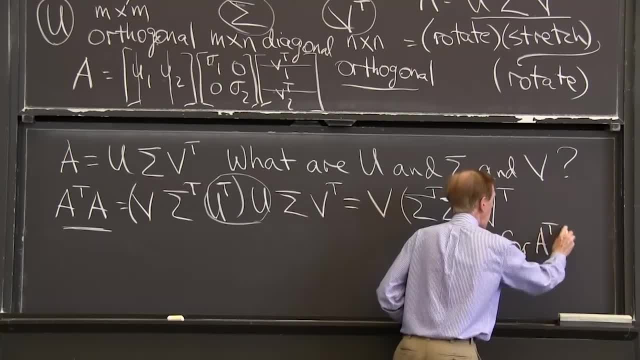 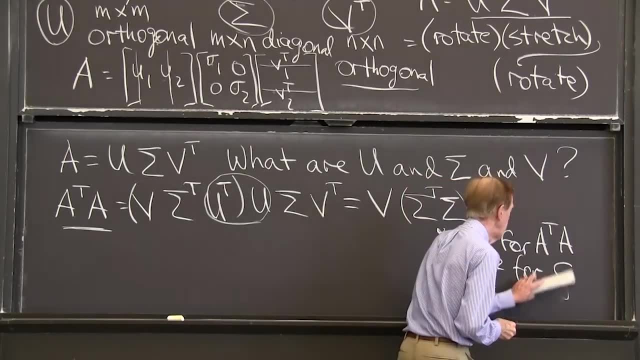 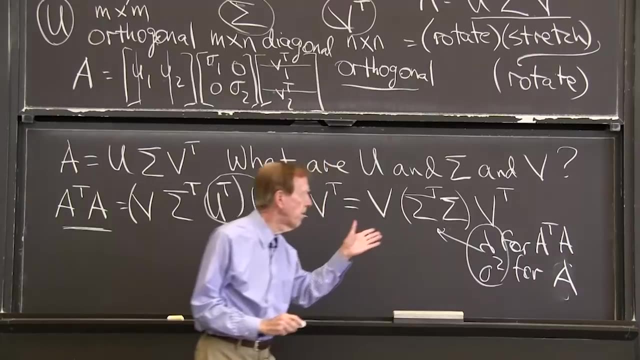 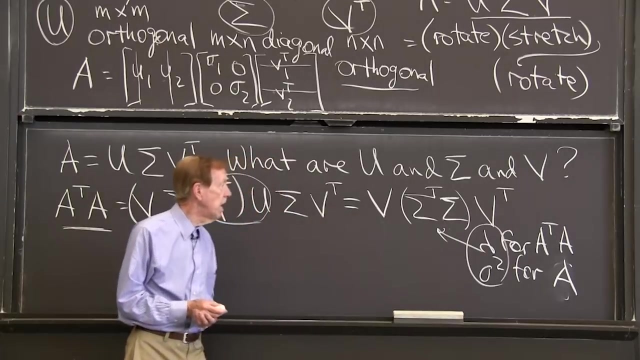 Lambdas for A transpose A are the sigma squareds for S, for A, for A itself, Lambda is the same. Lambda for A transpose A is sigma squared for the matrix A. All right, Well, that tells me v, That tells me sigma. 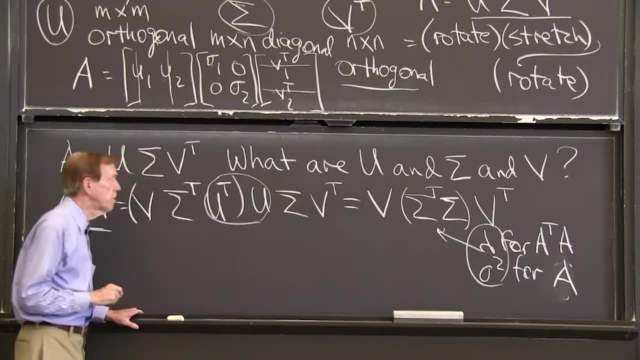 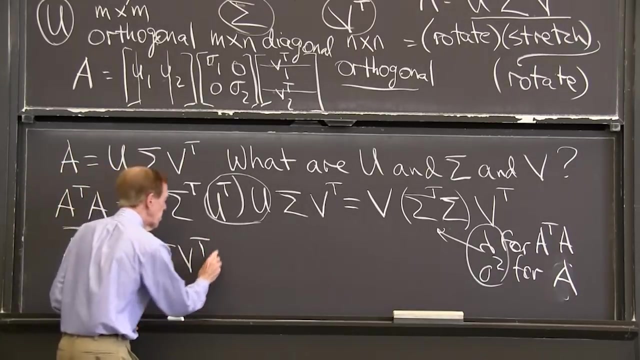 And you disappeared here Because u transpose. u was the identity. It just went away. How would I get hold of u? Well, here's one way to see it: I multiply A times A transpose in that order, In that order. So now I have u sigma v- transpose, times the transpose. 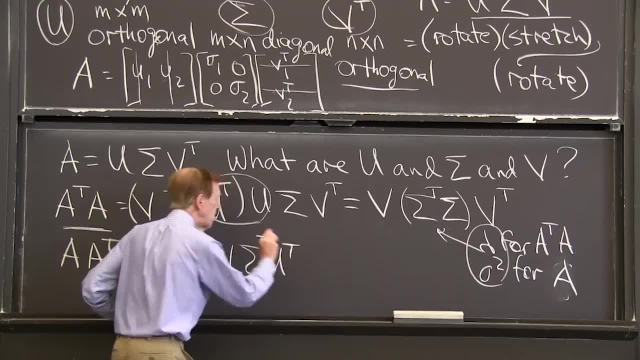 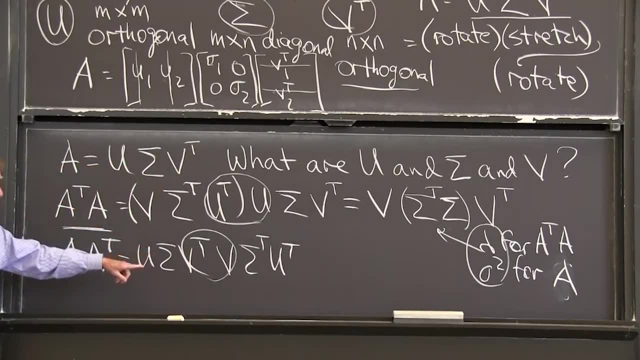 which is the v sigma: transpose, u transpose. I'm having a lot of fun here with transposes, But v- transpose, v is now the identity in the middle. So what do I learn here? I learn that u is the eigenvector matrix for A- A transpose. 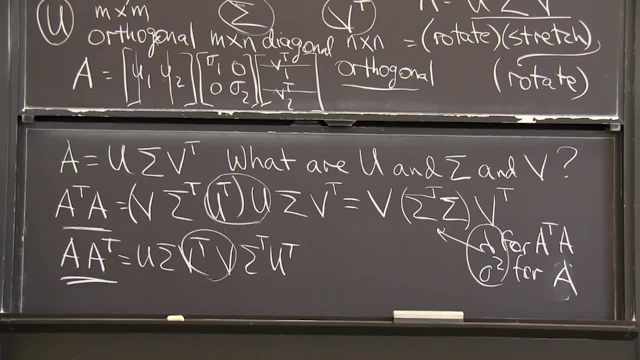 So these have the same eigenvalues. A times B has the same eigenvalues as B times A. In this case it comes out here: Same eigenvalues. This has eigenvectors v. This has eigenvalues. This has eigenvectors u. 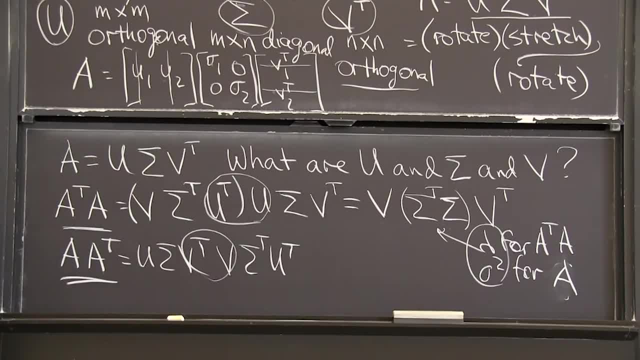 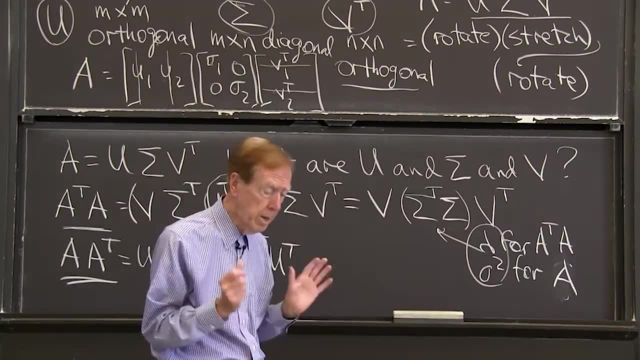 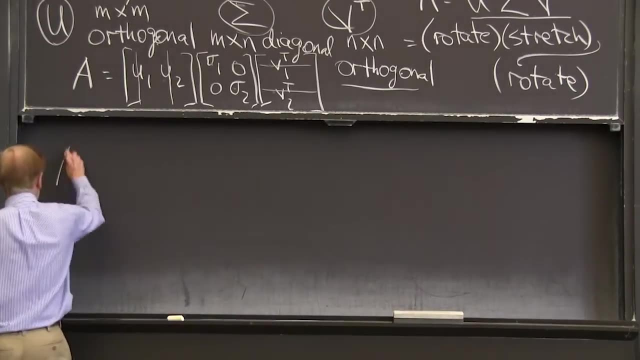 And those are the v and the u in the singular value decomposition. Well, I have to show you an example. I have to show you an example and an application, And that's it OK. So here's an example. Suppose A: I'll make it a square matrix: 2, 2, minus 1, 1.. 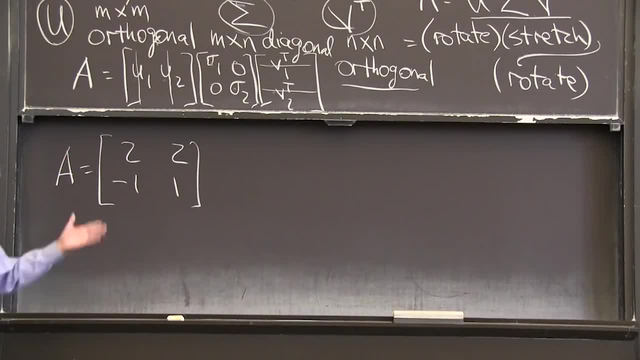 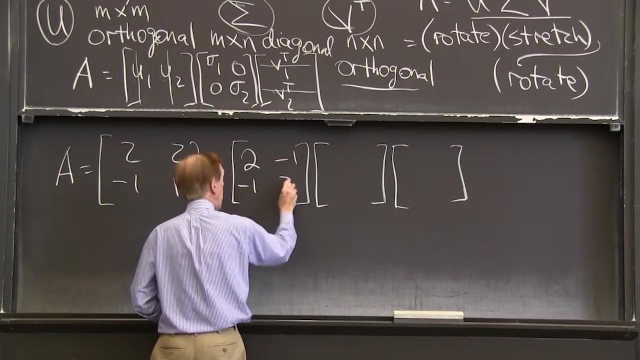 Not symmetric, Certainly not positive definite- I wouldn't use the word Because that matrix is not symmetric, But it's got an SVD, three factors And I work them out. This is the orthogonal matrix. I have to divide by square root of 5 to make it unit vectors. 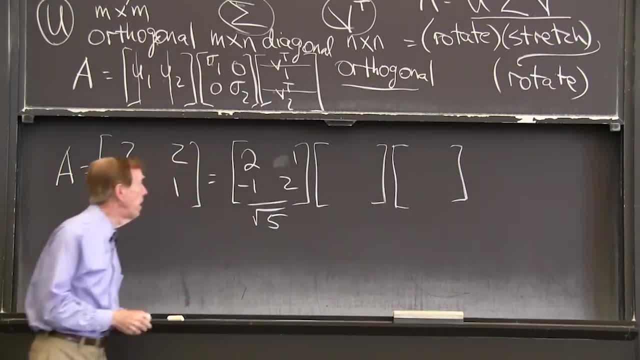 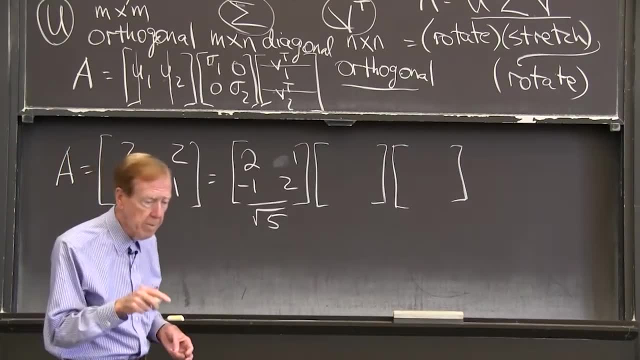 Oops, that's not going to work. How about that? The two columns are orthogonal, And that's a perfectly good u. And then in the sigma, I got. well, that's a. oh, I did want 1 and 1.. 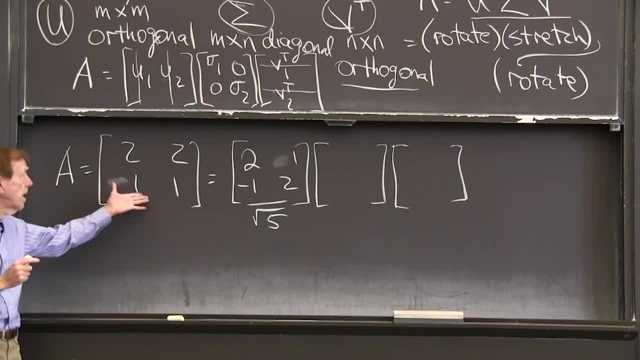 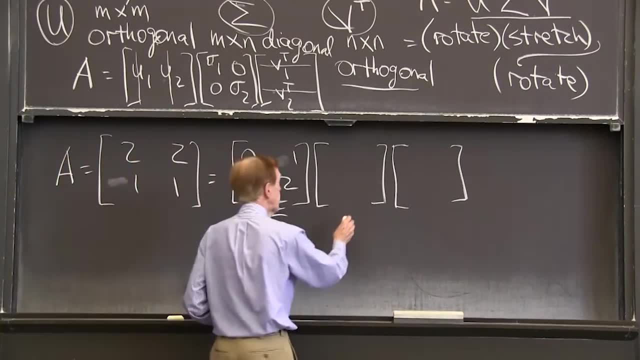 I did want 1 and 1.. Yes, Ah yes. So I have a singular matrix, Determinant 0, singular matrix, So my eigenvalues will be 0.. And it turns out, square root of 10 is the other eigenvalue. 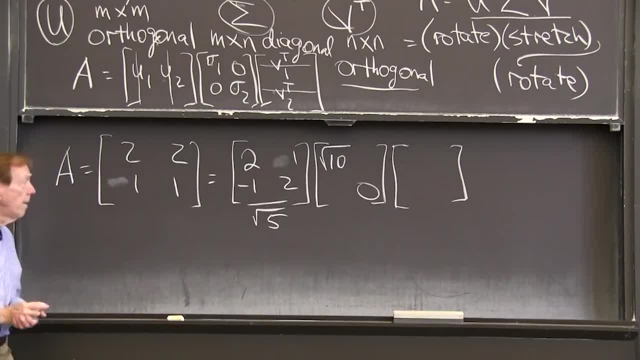 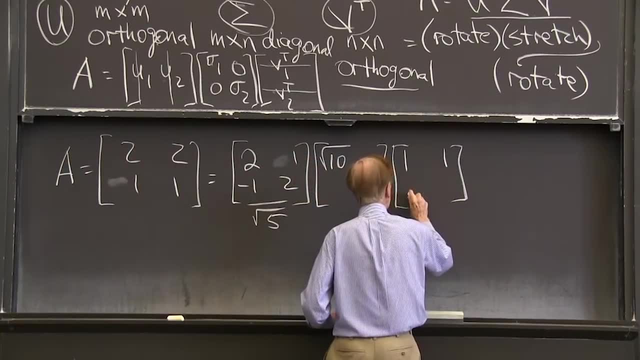 for that Other singular Singular value for this guy. And now I'll put in the v transpose matrix, which is 1, 1.. And 1 minus 1, is it? And those have lengths, square root of 2,. 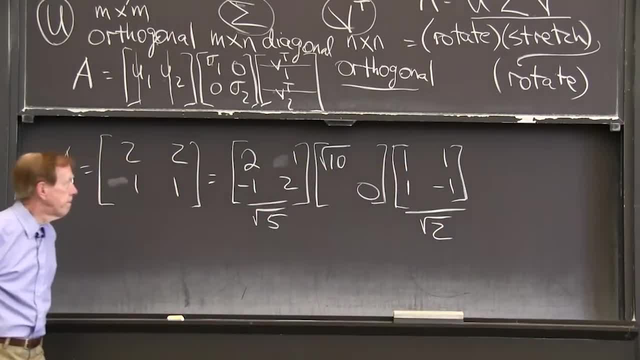 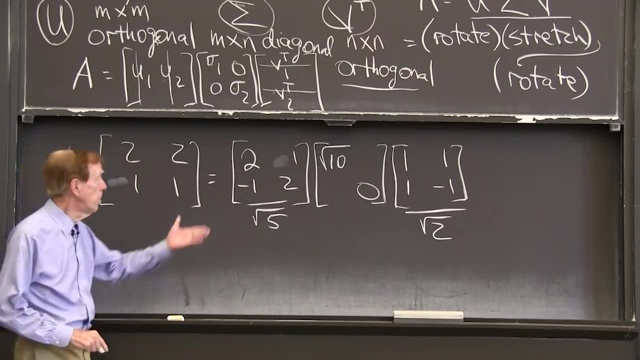 which I have to divide by. Well, I didn't do that so smoothly, but the result is clear: u sigma v transpose. So here's the sigma, And the singular values of this matrix are square root of 10 and then 0.. 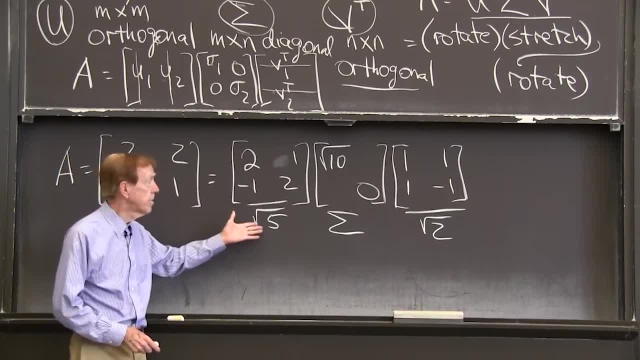 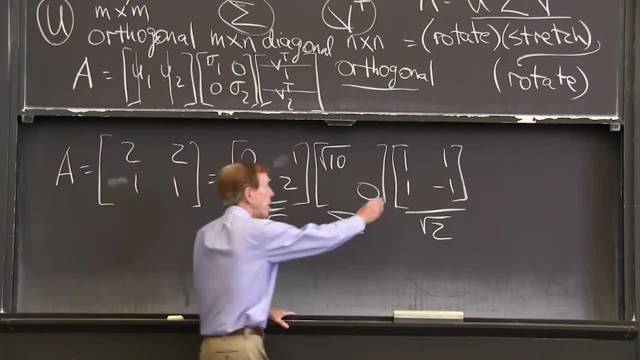 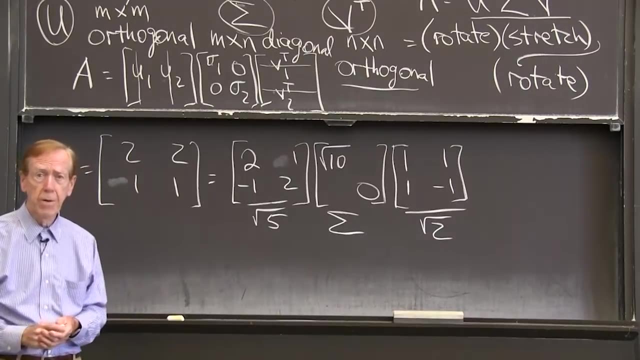 Because it's a singular matrix. And the eigenvectors? well, the singular vectors of the matrix are the left singular vectors and the right singular vectors. OK, That looks good to me. And now the application. to finish, A first application is well, very important. 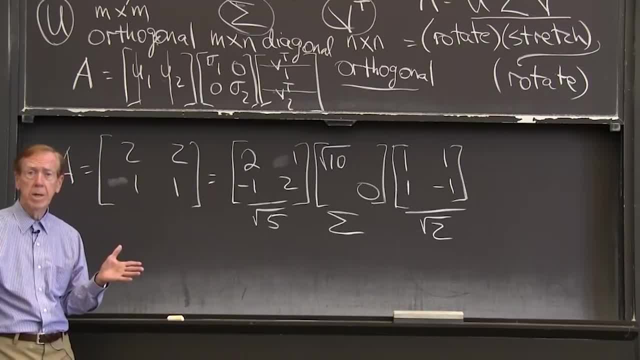 All the time in this century we're getting matrices with data in them. Maybe in life sciences we test a bunch of samples, people for genes. So I have a. my data comes somehow. I have a gene, I have a matrix. 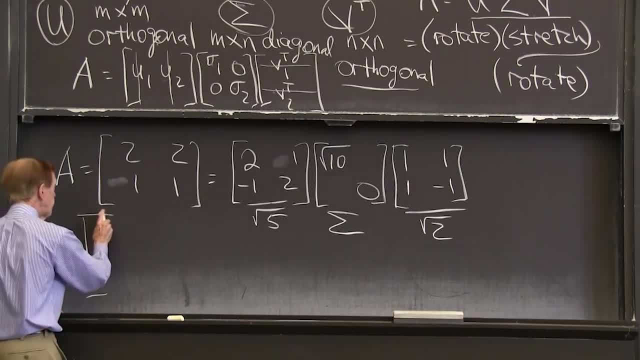 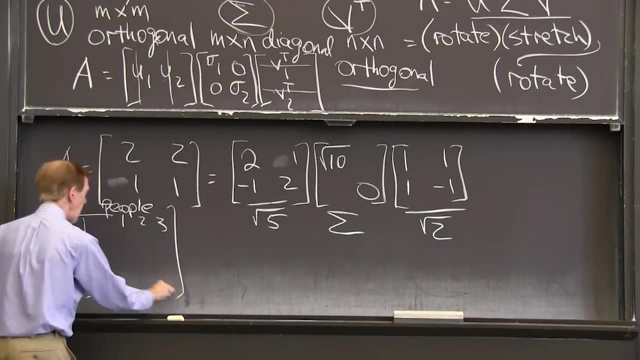 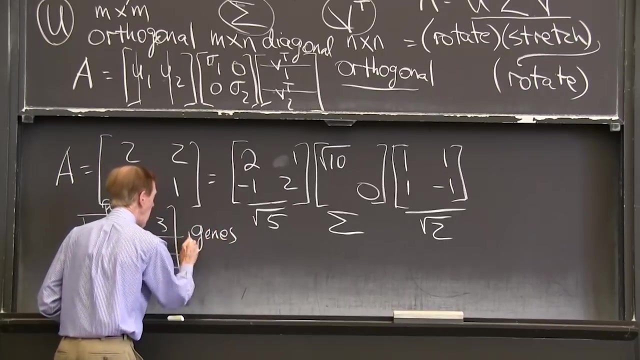 I have a gene expression matrix. I have samples, people, People 1,, 2,, 3 in those columns And I have in this in the rows, let me say, four rows. I have genes, gene expressions That would be completely normal. 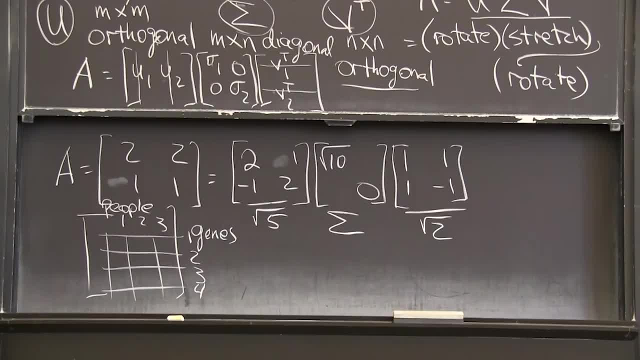 A rectangular matrix because the number of people and the number of genes is not the same And in reality those are both very, very big numbers. So I have a large matrix And out of it I want to and each number in the matrix. 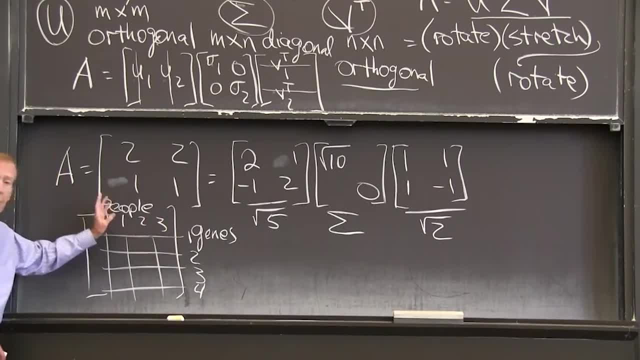 is telling me how much the gene is expressed by that person. We may be searching for genes causing some disease. So we take several people, some- well, some- with the disease, We check on the genes, We get a big matrix And we look to understand something out of it. 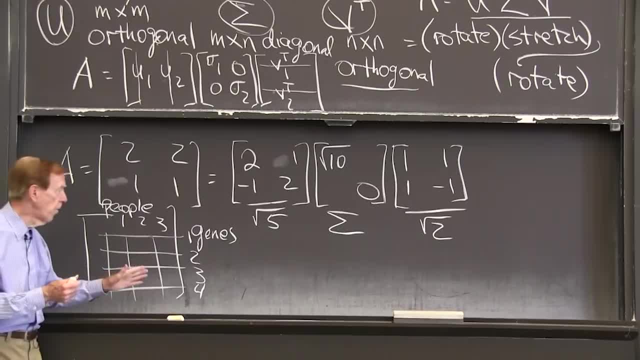 What can we understand? What are we looking for? We're looking for the correlation, the connection between some combination maybe of genes and some. we're looking for a gene-people connection here, But it's not going to be person number one. 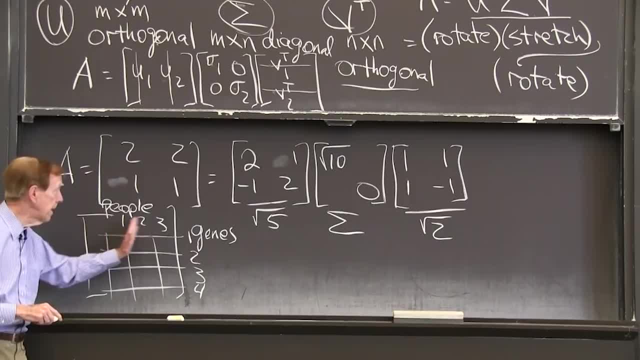 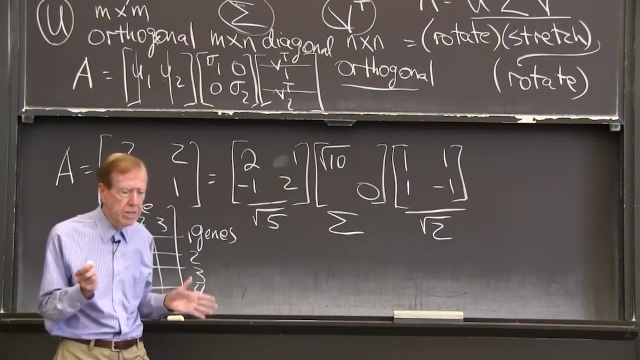 We're not looking for one person, We're going to find a mixture of those people. So we're going to have sort of an eigen-sample. eigen-people- Oh, that's terrible. Eigen-person would be better. So I think I'm seeing an eigen-person. 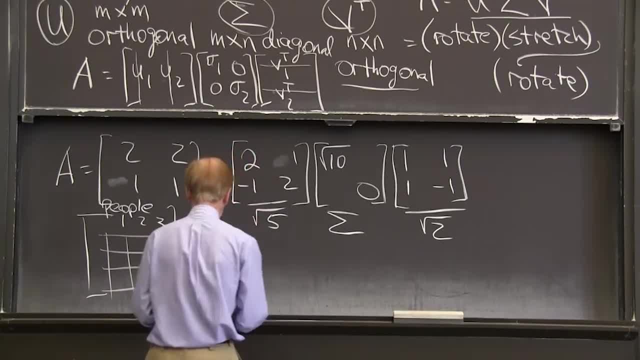 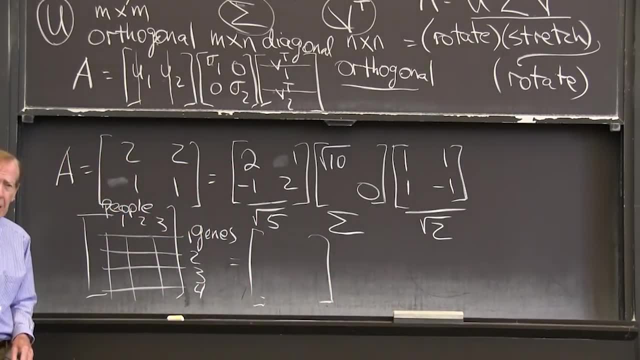 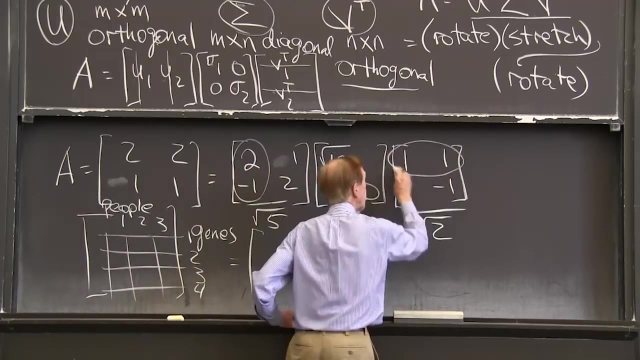 Let me see where I'm going to put this. So, yeah, I think my matrix would be written. Oh, here's the main point. That, just so you know That, just as I see in this example, it's the first vector and the first vector. 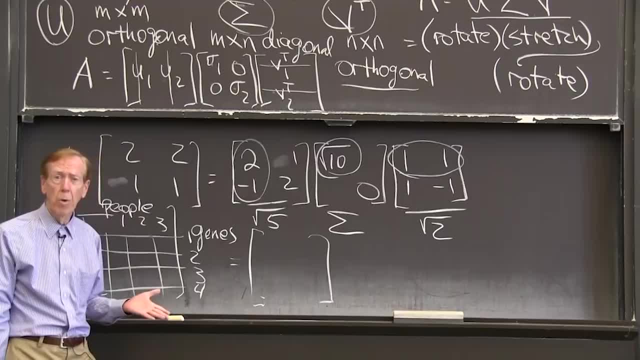 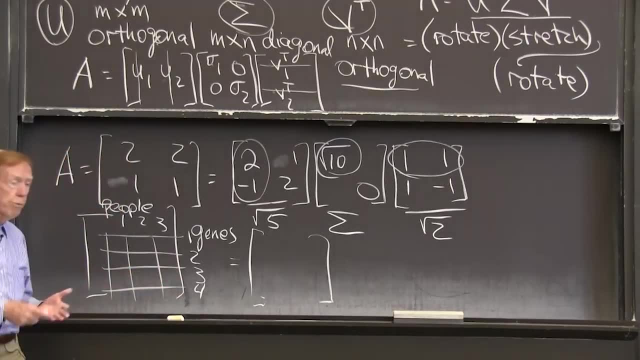 and the biggest sigma. that are all important. Well, in that example the other sigma was 0, nothing. But in this example I'll probably have three different sigmas, But the largest sigma, the first, the u1 and the v1,. 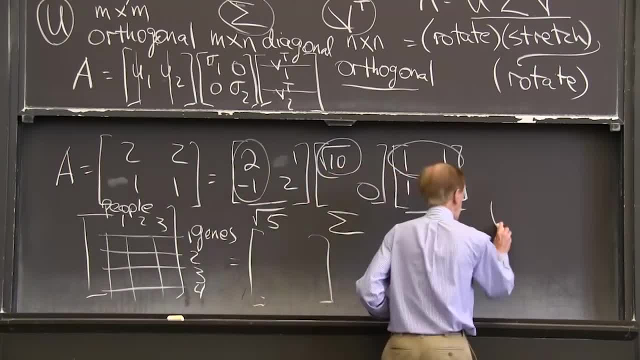 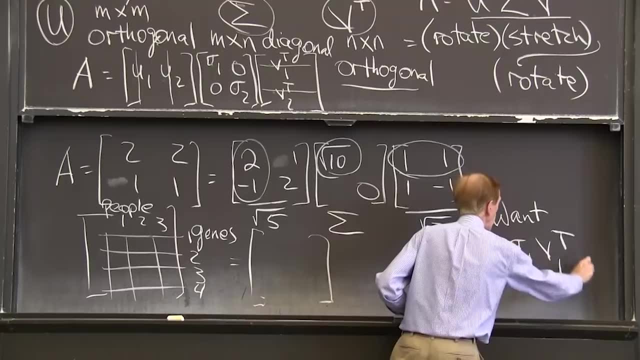 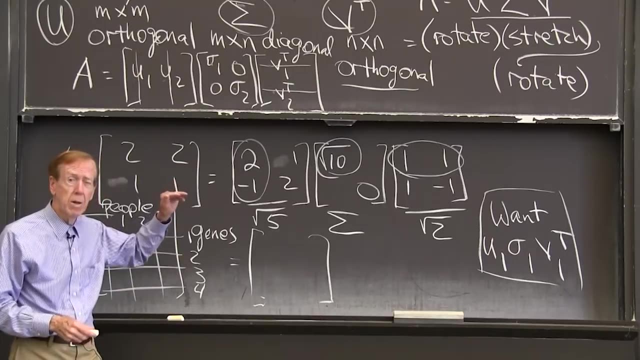 it's that combination that I want. I want u1, sigma 1, v1- transpose, the first eigenvector, of A transpose A and of A, A transpose. and the first singular, the biggest singular value, That's the information. 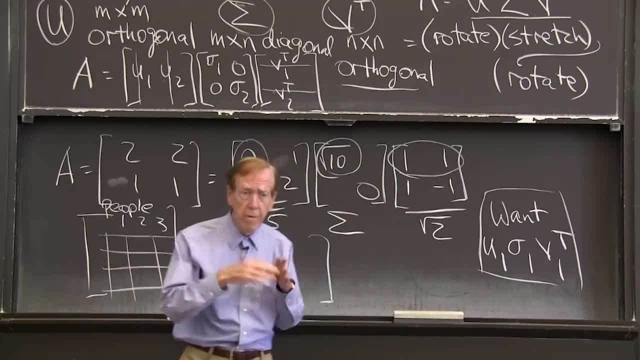 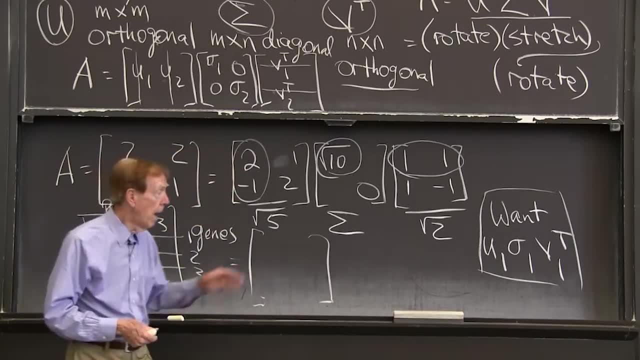 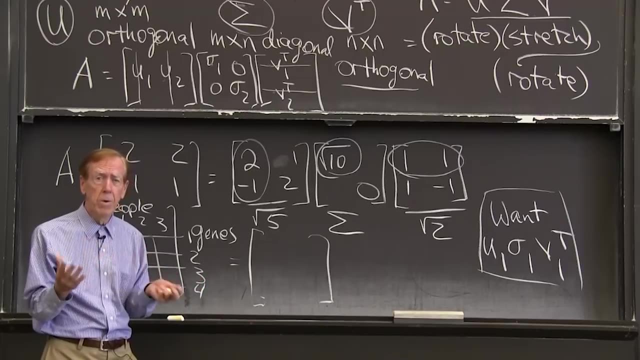 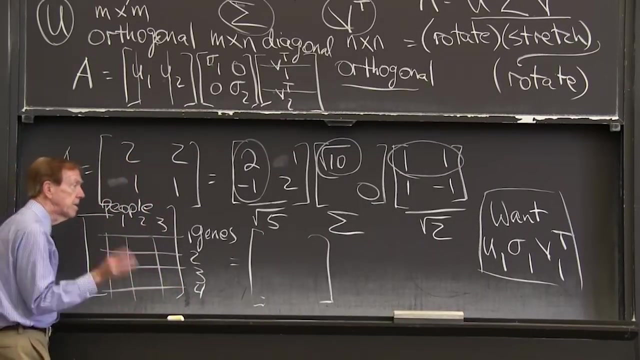 That's the best sort of put together, person, eigen-person combination of these people and the best combination of genes That has the in statistics I would say the greatest variance. In ordinary English I would say the most information, The most information in this big matrix. 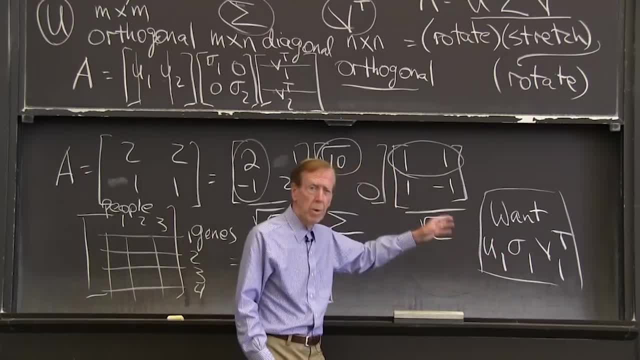 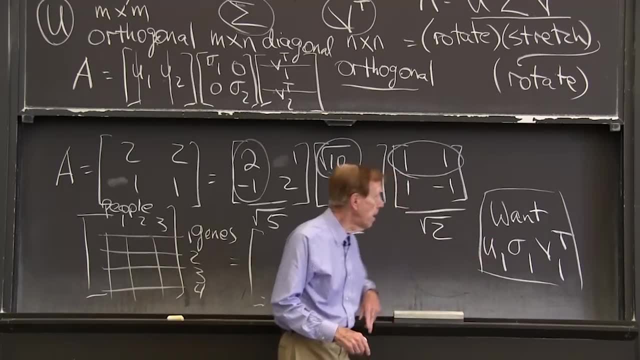 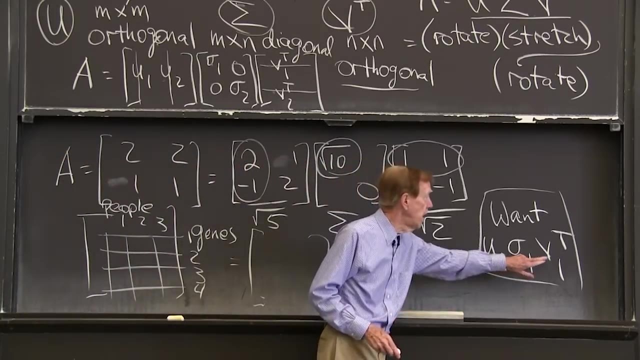 is in this very special matrix, with only rank 1, only a single column repeated, a single row repeated and a number sigma 1, the number that tells me that, Because u is remember, u is a unit vector. v is a unit vector. 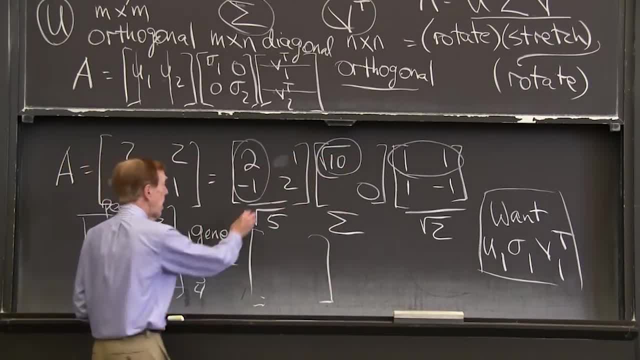 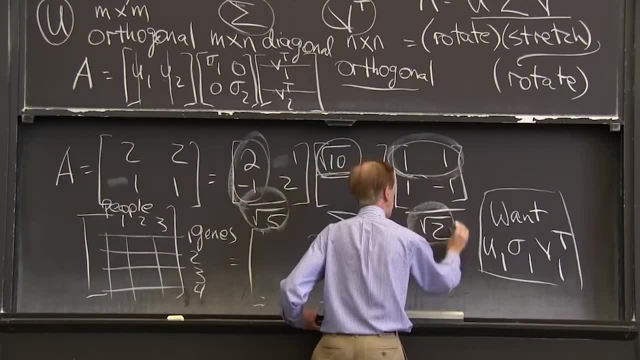 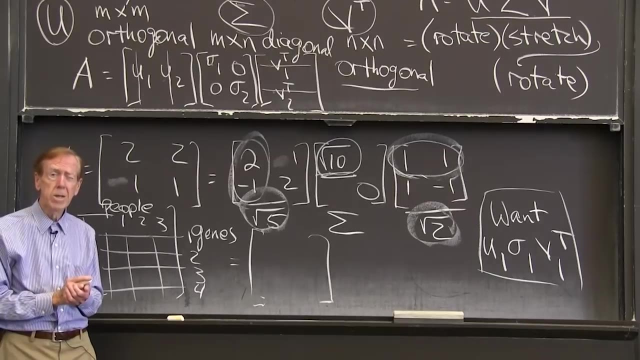 v is a unit vector. It's that number sigma 1 that's telling me. So it's like that unit vector times that number. key number times that unit vector. I'm talking here about principal component analysis. I'm looking for the principal component, this part.